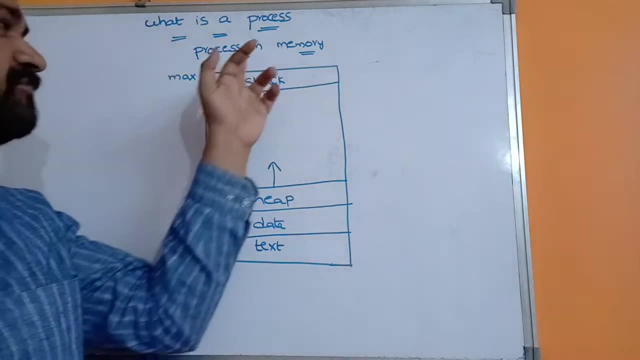 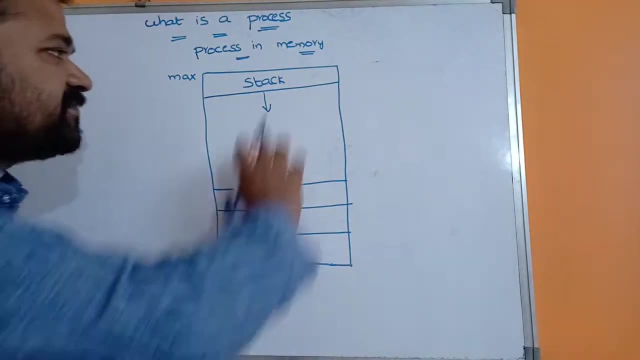 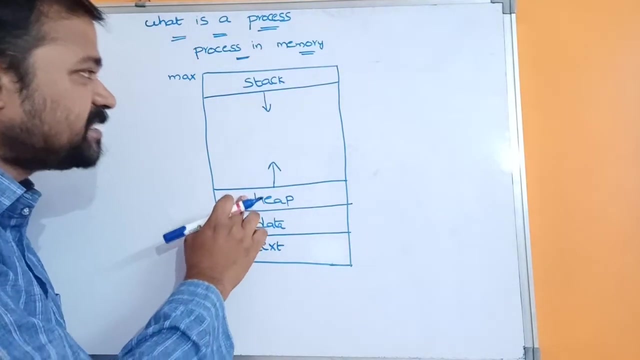 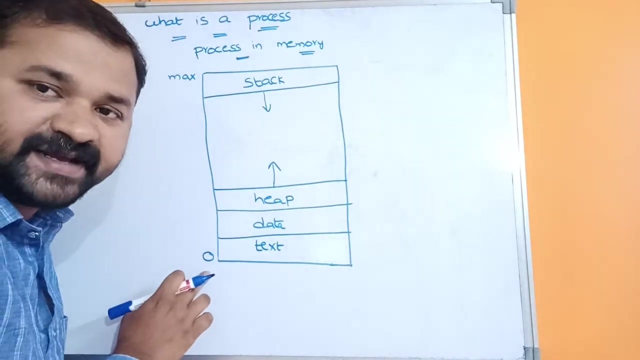 memory. only now let's see this diagram. every process is represented internally in main memory in this format. so here we have several segments. the first segment is text segment, next one data segment, next one heap segment, next one stack segment. here these are nothing but address locations, the minimum address. 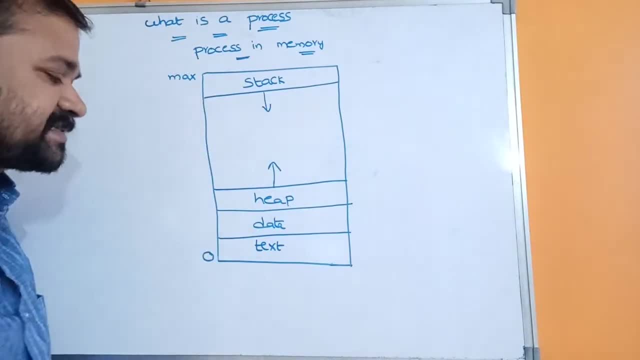 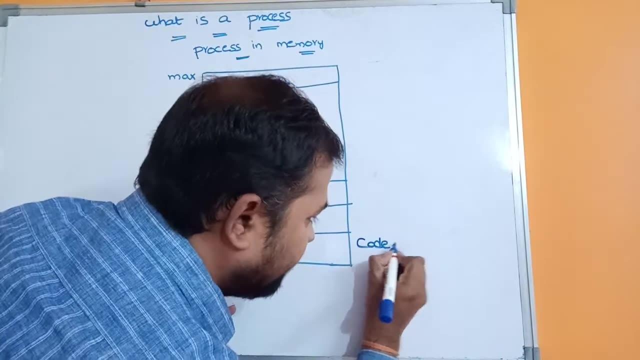 segment is the address location and the minimum address location is the data is 0, whereas the maximum address is a max. first let's see what is text segment. text segment can also be called as core segment, so the other name for the text segment is core segment- text segment. 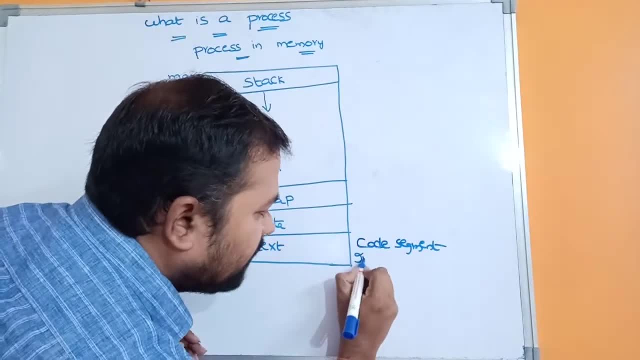 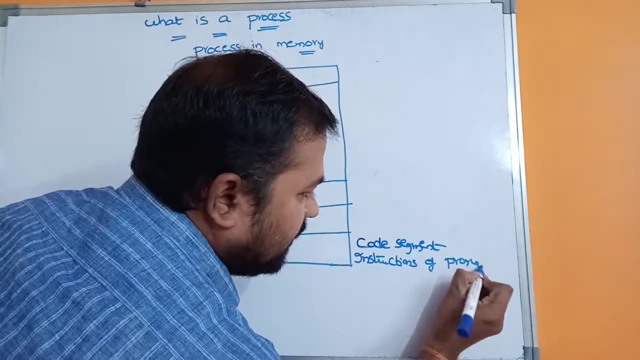 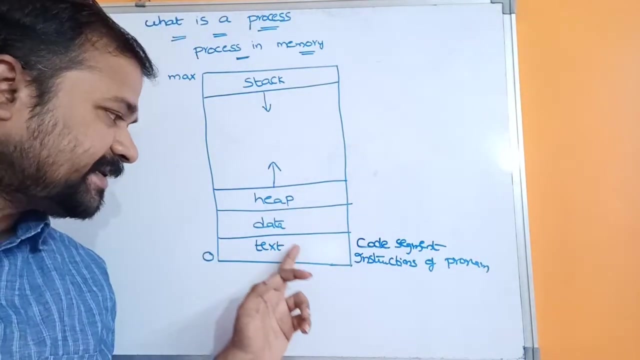 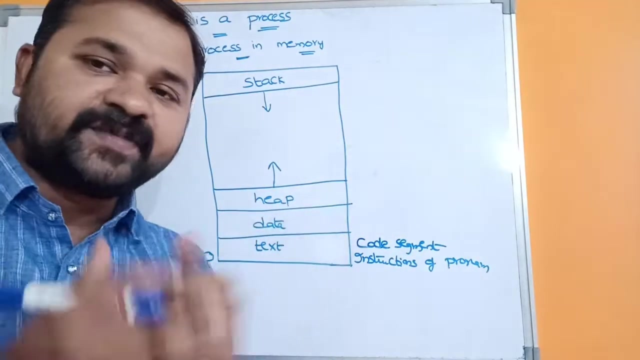 mainly stores program. so every program contains several instructions, so it stores instructions of the program. let the program contains 10 statements, 10 instruction, so those 10 instructions will be stored in the text segment. what is the other name for text segment? code segment? now let's see what is data segment. it mainly stores global variables as well. 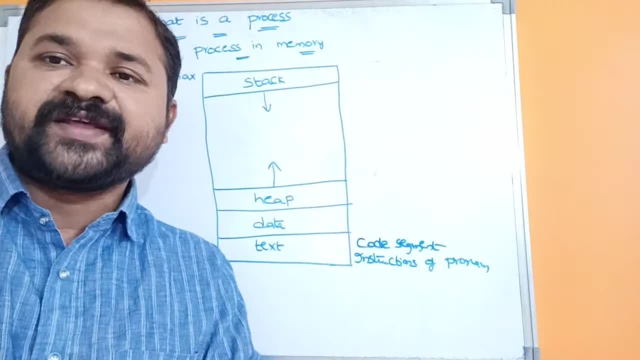 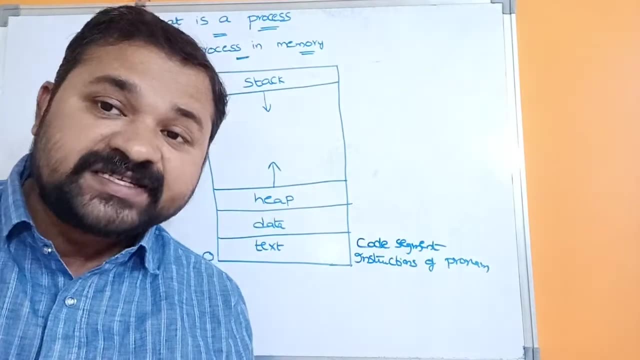 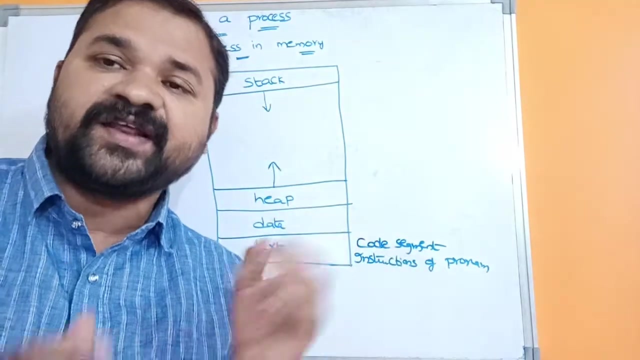 as static variables. we know what is a global variable. global variable means we can use that variable throughout the program, so that we have 100 functions in the program. if you want to use a common variable in all the 100 functions, then we can make use of global variable, and we know. 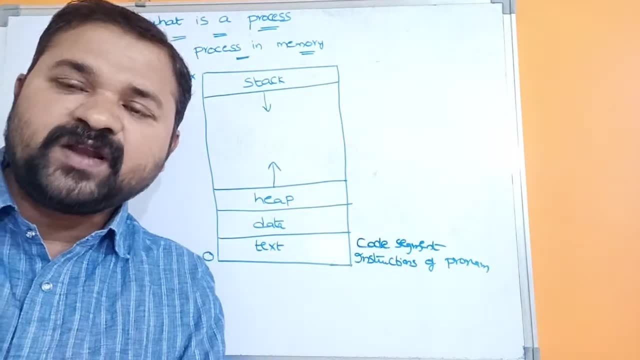 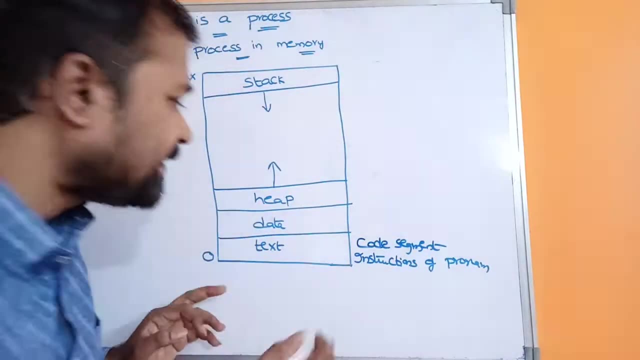 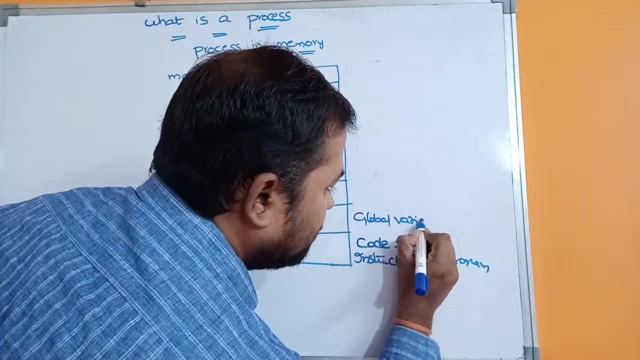 about static variable. for static variable, the memory will be created only once and all the functions will make use of that variable. okay, so data segment is mainly useful in order to store global variables as well as static variables- global variables as well as static variables. so if there are any global variables and 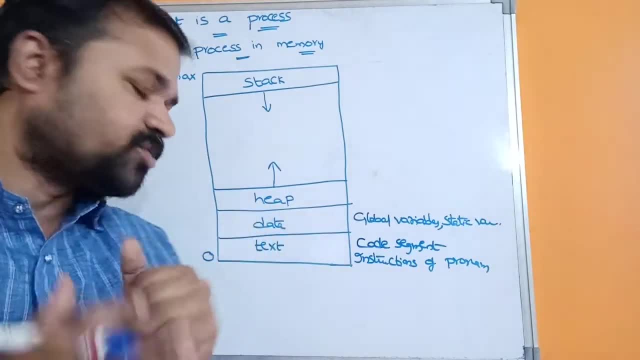 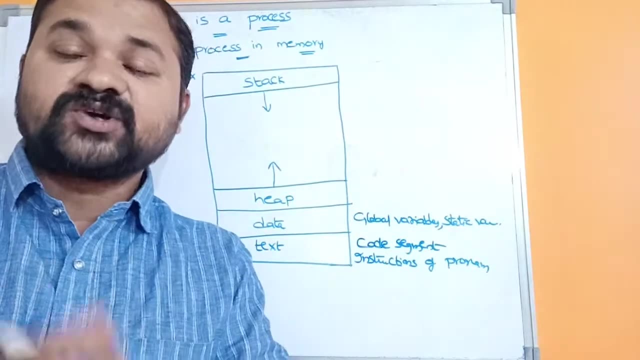 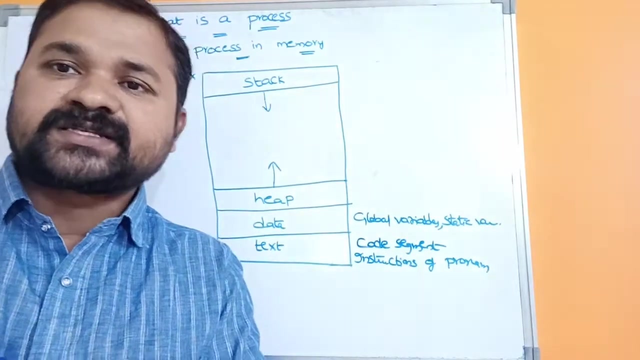 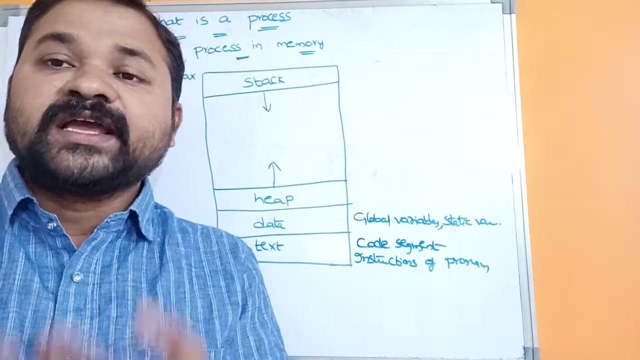 static variables in our program, then those variables will be stored in data segment. okay, and the next one is heap segment. we know what is dynamic memory allocation. so dynamic memory allocation means allocation of memory during runtime. generally, for pointers, the memory will be allocated during runtime. so here heap section is mainly useful in order to store variables. 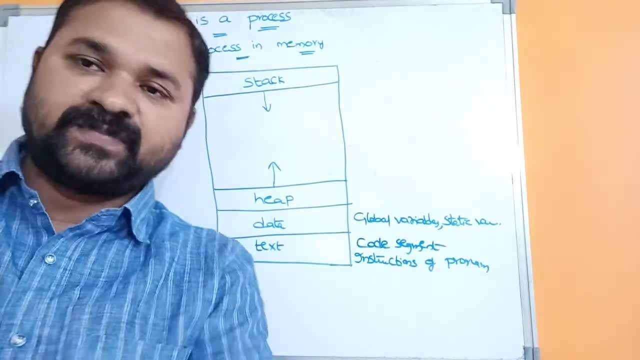 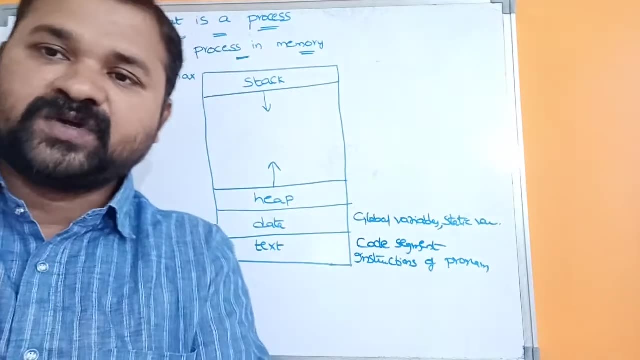 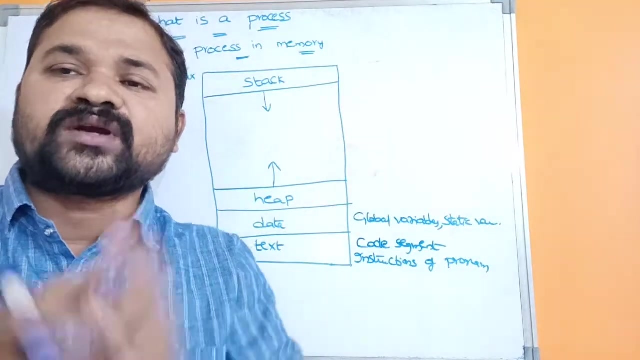 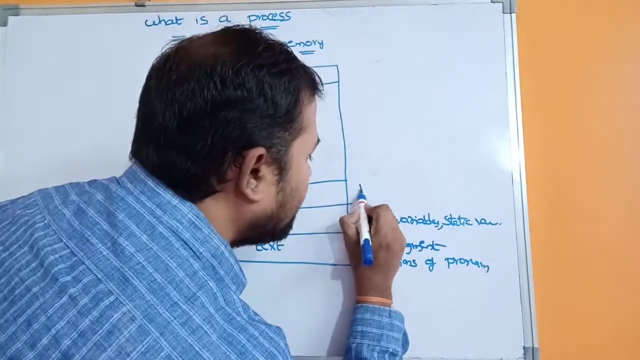 whose memory was allocated during runtime. so let we have two pointers. so for those two pointers the memory was allocated during runtime, so those variables will be stored in the heap. so heap is mainly useful in order to store dynamically memory allocated variables. okay, so why we are using heap here? it is useful in order to store dynamic, dynamic memory. 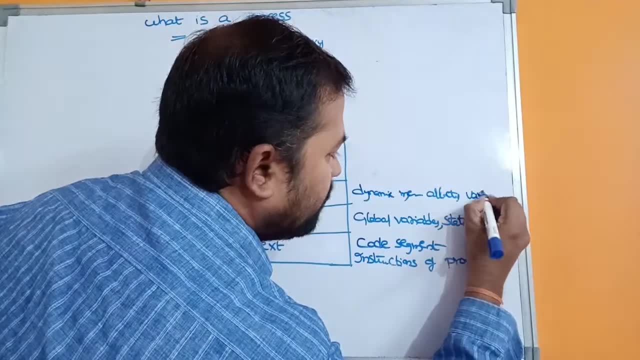 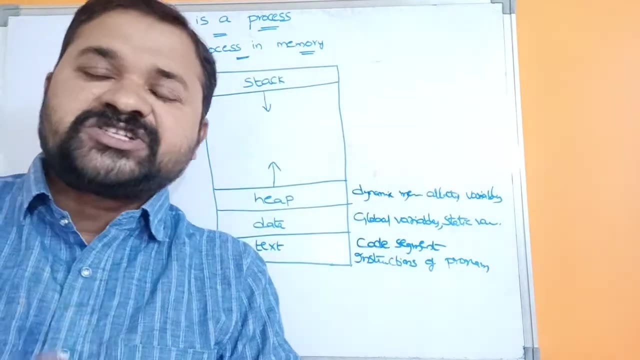 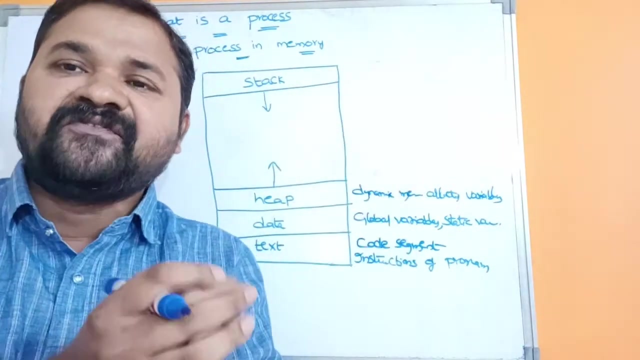 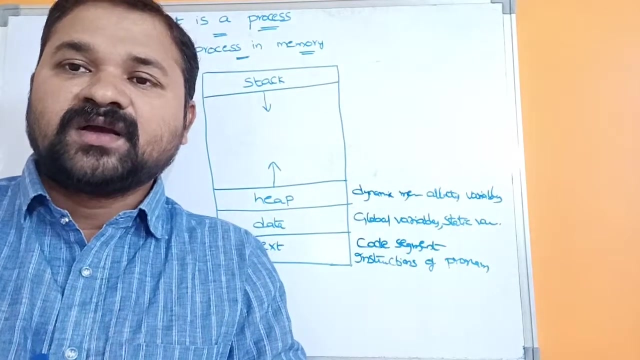 allocated variables, dynamic memory, allocated variables. okay, and here we have one more section, that is stack section. stack section is nothing, but it is also called as function stack. so here we are using stack mainly while calling the function. so whenever we call a function, then the function should contain some parameters as well as function should contain within the. 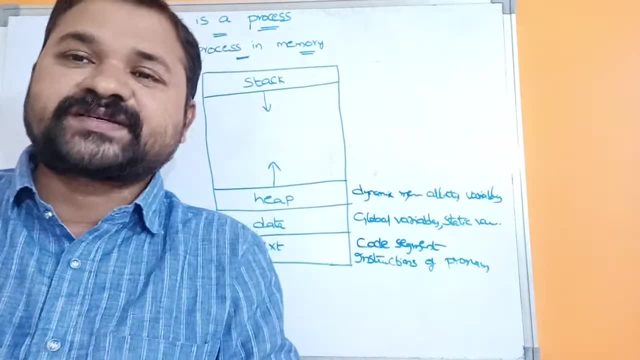 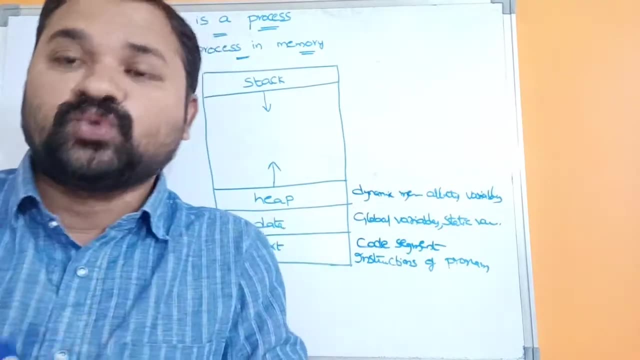 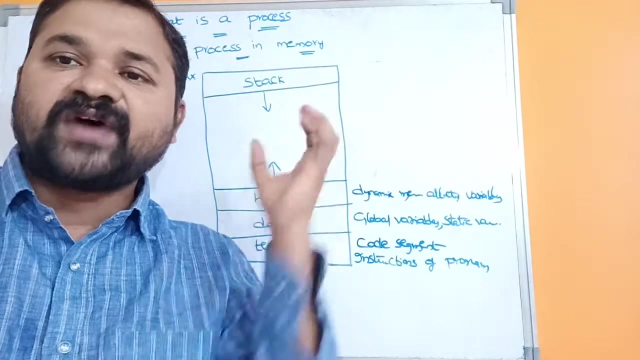 function. we can have some local variables, some temporary variables, some temporary variables. we can use those local variables or temporary variables in that function only as well as it should retain some value. okay, so all those parameters will be stored in the stack. so what is the other name for stack function? stack? so why we are using stack. stack is mainly useful. 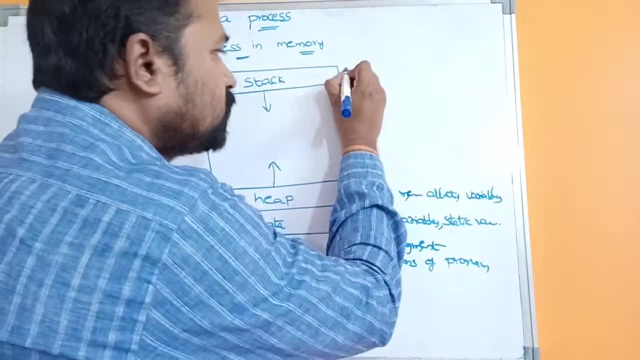 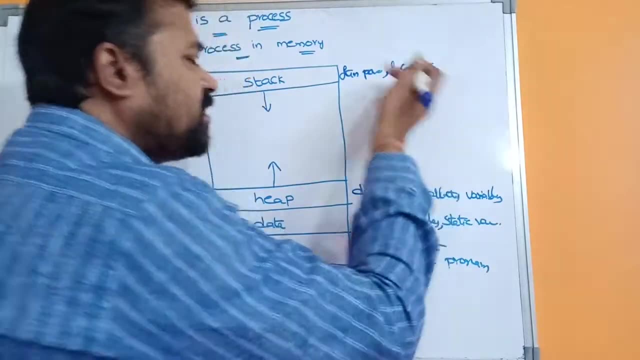 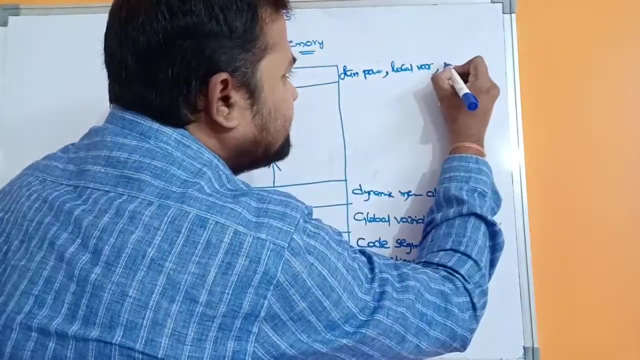 in order to store function parameters. so we can store the function parameters as well as local variables. these local variables can also be known as temporary variables. why? because we can use those variables only inside that function as well as if it returns any variable, okay, that return variable. okay, that return variable can also be stored with the. 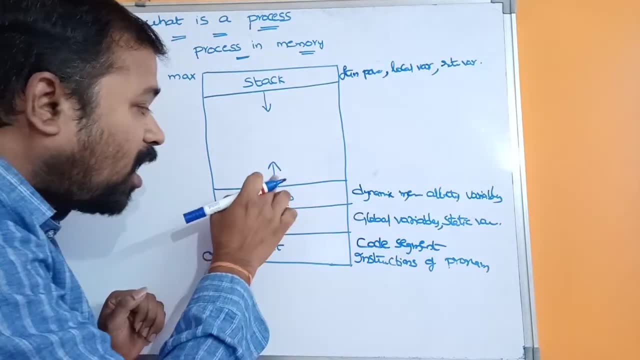 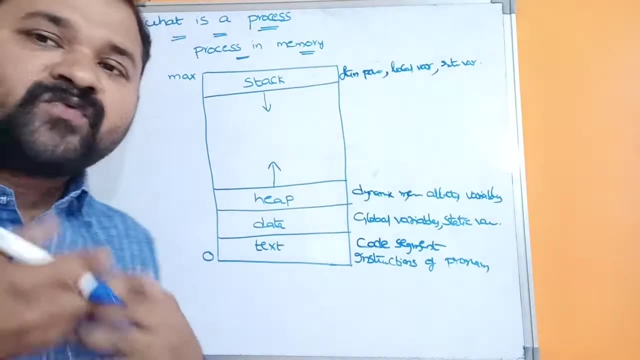 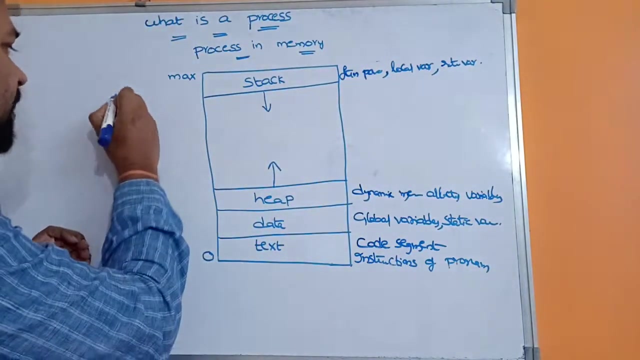 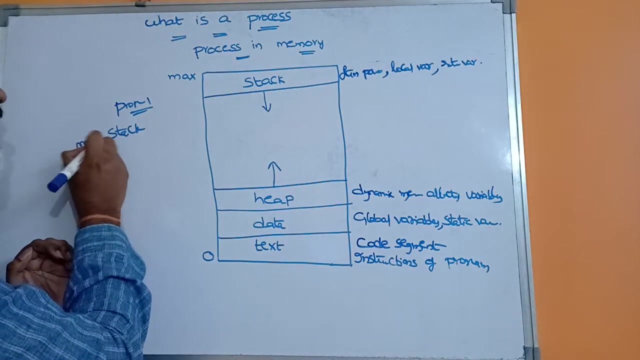 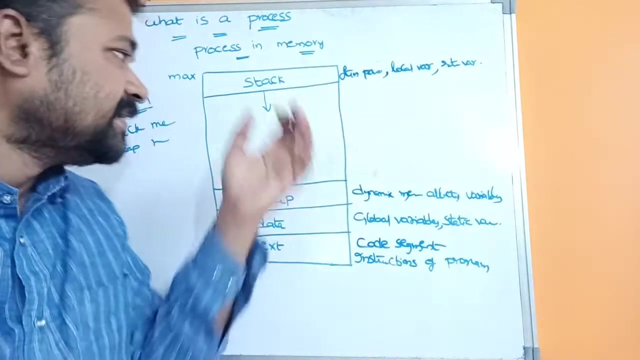 help of the stack. here, heap always grows upside, whereas stack always grows downside. why? because we don't know which segment will use us more memory. let us assume that we have a program called program one. in program one, we are using more stack memory, more stack memory as well as less heat memory. so in that occasion, what will happen is stack will make use of more. 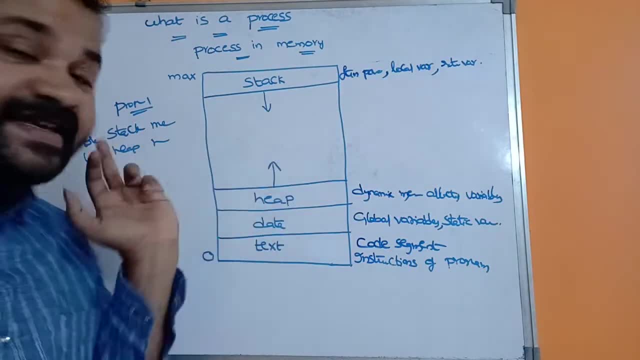 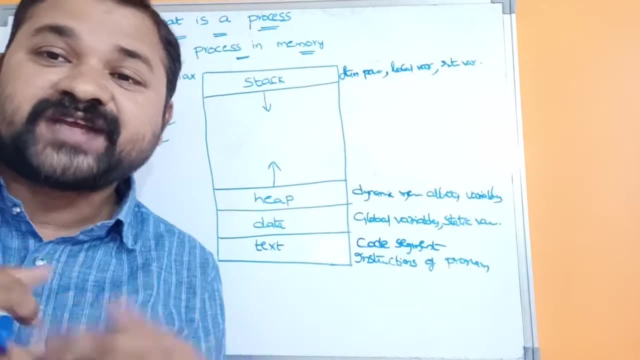 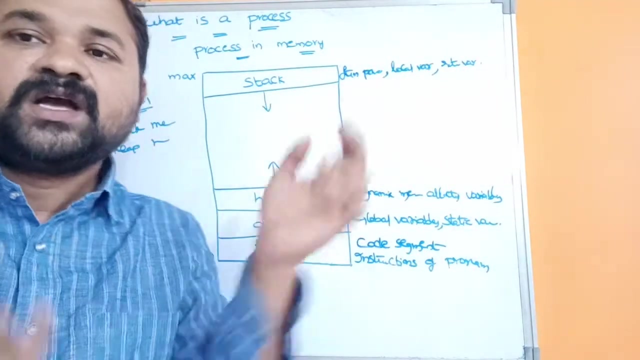 memory as well as heap will make use of less memory, so that's why we should not split the stack and heap. okay, so depends upon the stack and heap they will share. let us assume that in certain program, heap memory is very, very high, whereas stack memory is very, very less. okay.